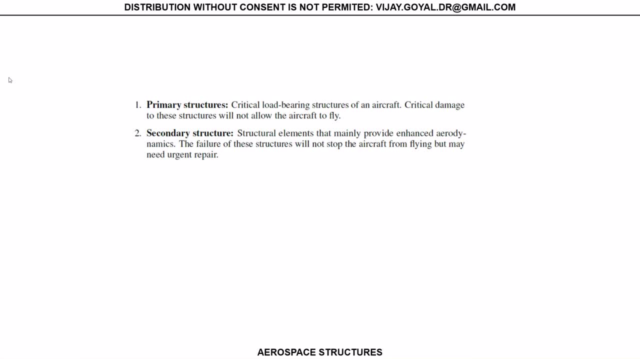 to carry most of the load. A secondary load path is one that may not necessarily carry the major load. As for an example, if I design, if I put two spars like this right, and these are spars, so you could design them, maybe something like this: these are spars, this is a c channel spar. 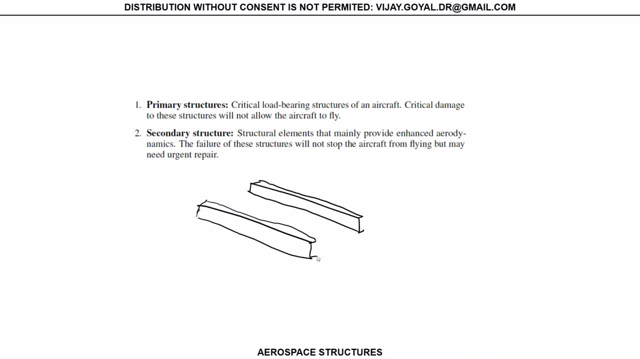 and now I design my plane on top of these spars. I place like I put some skin on top of it. right, if I can get this right, something skin, and this is kind of your airfoil and it goes like this. so, and then also you have here: 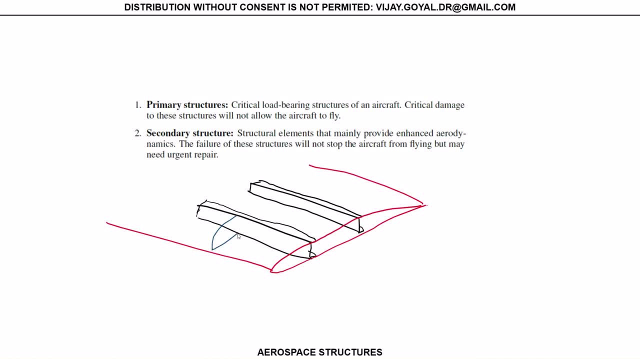 you can have ribs. uh, ribs are attached here, so you got ribs here and you got ribs there, right? so these are ribs. typically, they are full of holes and so this is your structure, this structure, right here. this structure, this structure, this structure is the main, the main loading structure. 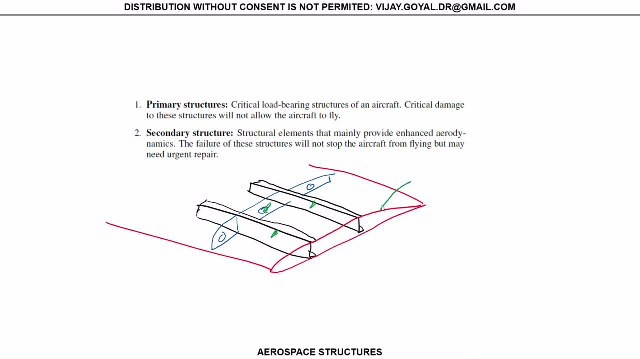 now you have a secondary loading structure. that would be your wing, that would be your skin. you could have maybe a stringer that's attached to the, a small stringer that's attached to the, the wing itself, the, the skin itself. many times when you look- if I look from the side, you will see that you got your spar and then you have what you call a. 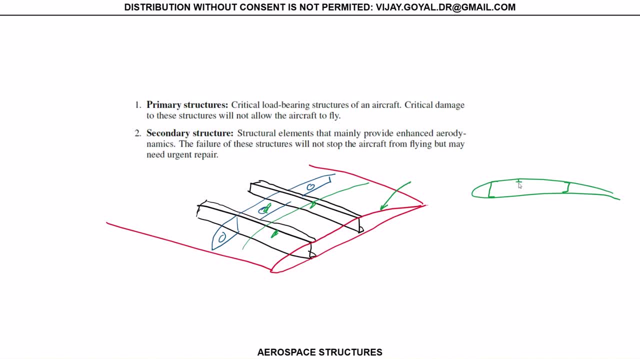 t string, a stringer that will go there and that is just a a, a low path that I create to help for my help, for stability purposes of the panel itself. so it's important when I'm designing something to know what I can. if something is going to fail, I will most likely want it to fail in a secondary. 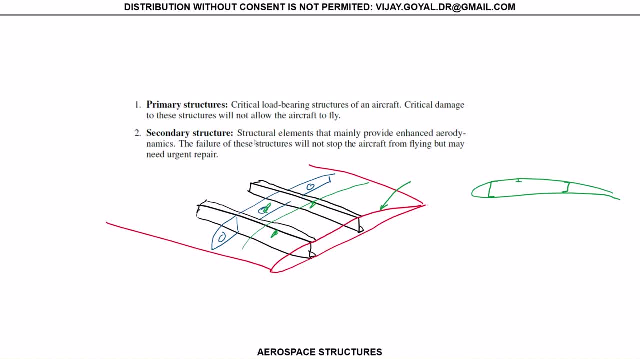 load path than the primary load path. you can think that if I lose one of these spars, if I lose this spar itself- now this spar doesn't exist- the possibility that this whole thing is going to collapse are huge, because this is what's really holding my entire aircraft in its place: my airfoil. 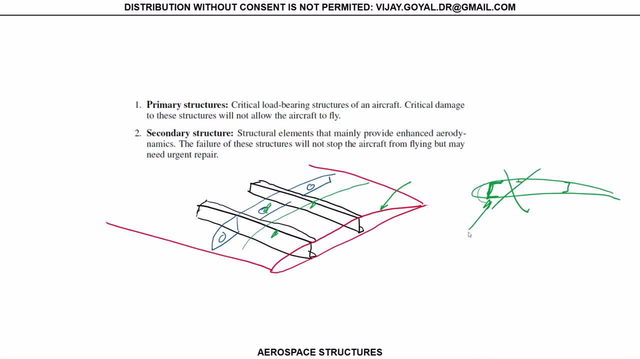 I'm sorry. so this, this part, cannot fail under no circumstances. neither can this. this is what we call a wing box is holding the whole wing box in its place, and a secondary load path and structure is okay. if it fails, at least I can land, my airplane will be able to land. 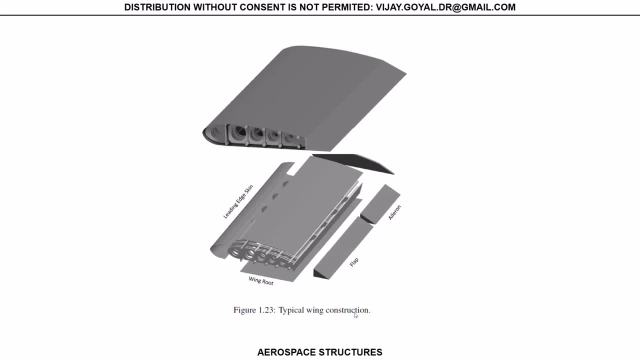 so, in a general, a typical wing, this construction- and this is for semi monocoque, we will talk about this later- mono coke, semi monocoque- is one that has skin. these are ribs, this represents stringers and these are the flaps and the. this is the wing root. so this is where your airplane is really. 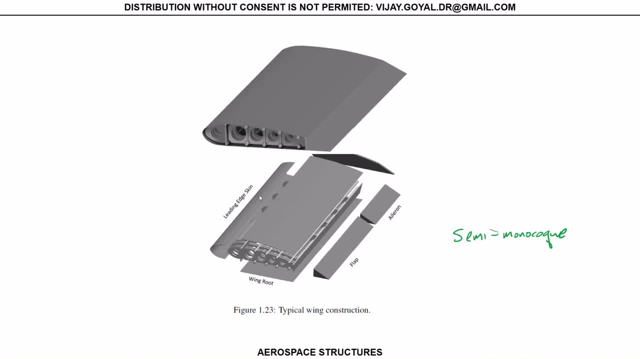 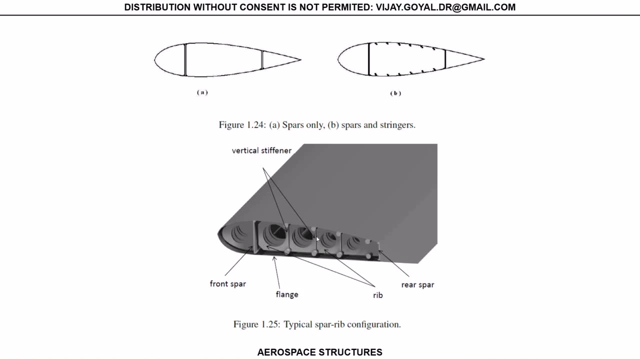 attached. so when you look at this whole thing here, this is the leading edge. this is more or less what it looks like. if I go a little bit more detail, you will see that this is what we call vertical stiffeners. this is what we call this front and rear spars. these are 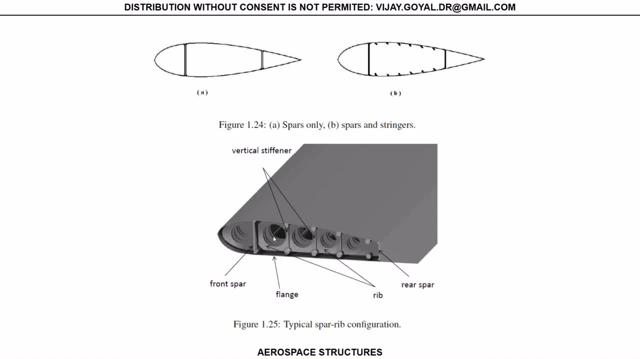 ribs right here, and the ribs have a purpose. why they got hole? the reason behind that they have holes is, first of all, make them light- lightweight. secondly, that's where your systems engineering is actually all the electricity, everything else that needs to be used, so you can see that there are a 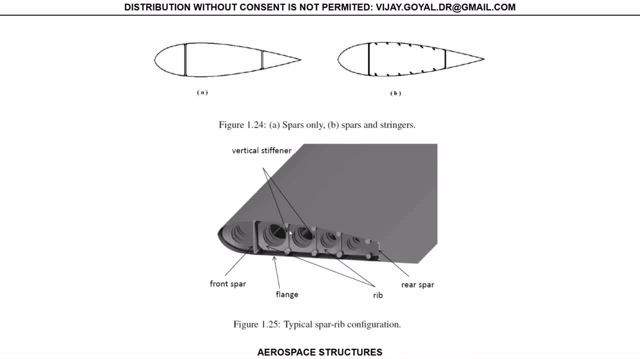 lot of holes that need to be gone through for one spot to another. that's where they will be located at, but we designed this holes. we design how much the dimension of this holes can possibly be okay. so this is a case where you have a wing with only spar. only this is spar, only this is a case where 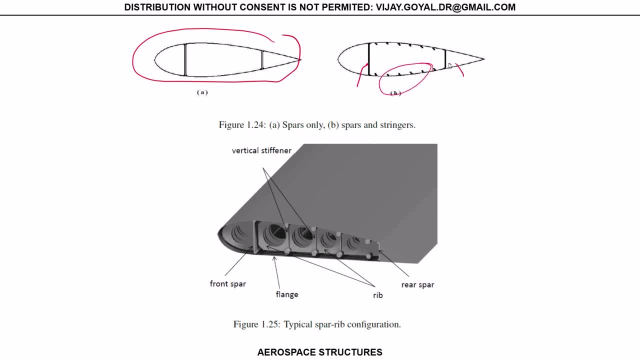 you got spar, you have a spar and you have stringers. okay, so this is mainly a monocoque construction, because it's saying that the entire structure- think about the wing, and I will make the wing as thick as possible and I want the whole, the whole structure to hold all the loads. as you can guess, this will be a heavier. 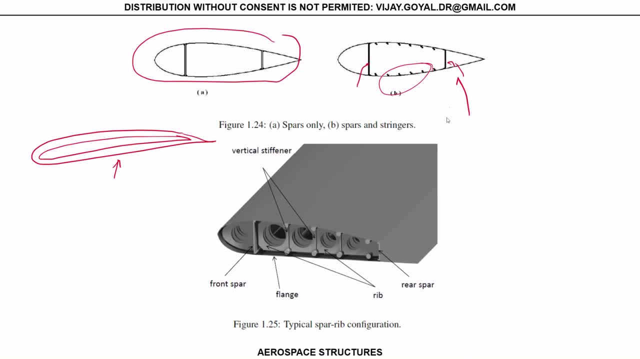 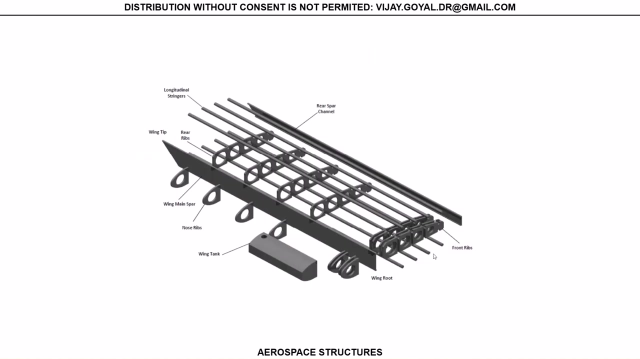 construction. but now, when I come to this, locate this part of the design, now I can say: this is only skin and this is what's really carrying most of my weight. so these are mainly the load-bearing main structures and everything else is secondary. um, this is a. if I just remove the skin, your it will look something like this: yeah, these. 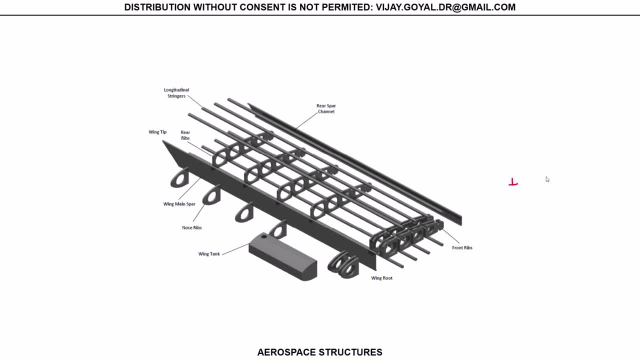 are not cylindrical, okay, they are sometimes T-shaped, sometimes L-shaped, uh, sometimes inverted. to you say, but this is where your skin is at top here, so they're all attached there, uh, so this is something like this so they can attach um, they attach with rivets, uh, or fasteners um your fuselage. 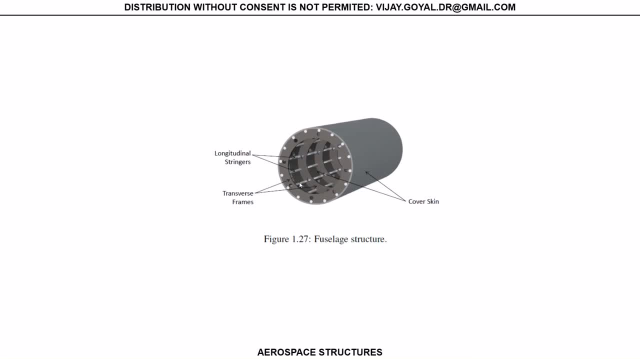 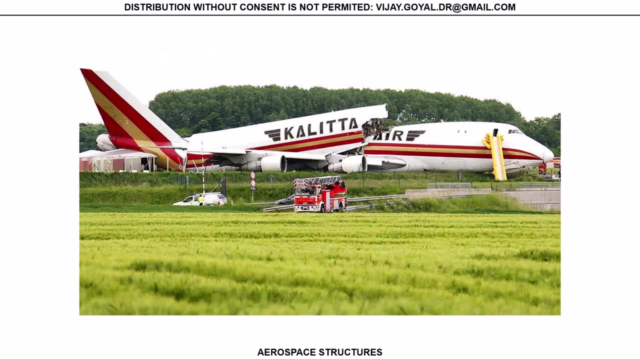 is a giant cylinder, uh, that basically has longitudinal stringers and also transfer frames. these are frames and this is the skin cover and what we want to study: airspace structures and I like to learn from history like, for instance, this particular airplane really just ripped apart right in the middle right, and as soon as it was landing, uh, and the landing processes as it ripped apart. 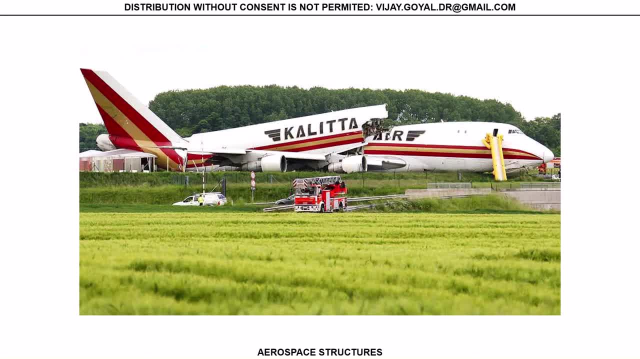 and if this is going to fail, like this typically fails, because it feels where the rivets are. and when I talk about rivets, it's basically: you got two panels, okay, and these two panels somehow are joined together and they are joined through rivets, okay. so underneath this you have something that 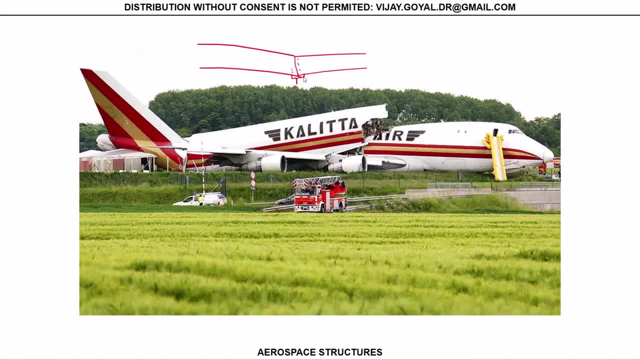 uh, join these panels together. uh, maybe a I-beam or a C-beam typically, and then so, if something good is going to break through the joints, um, and this is a very good example, in where you have not only failed through the joint but fell through the whole uh uh uh wing itself, and this is example as 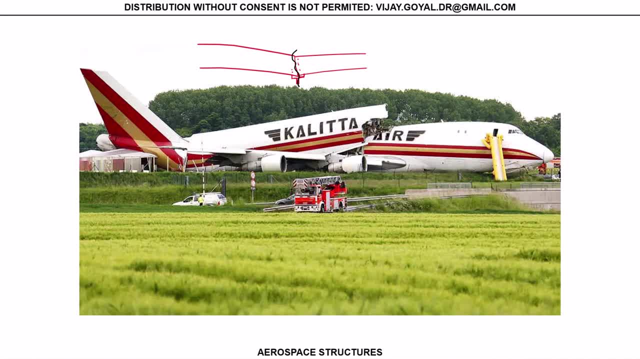 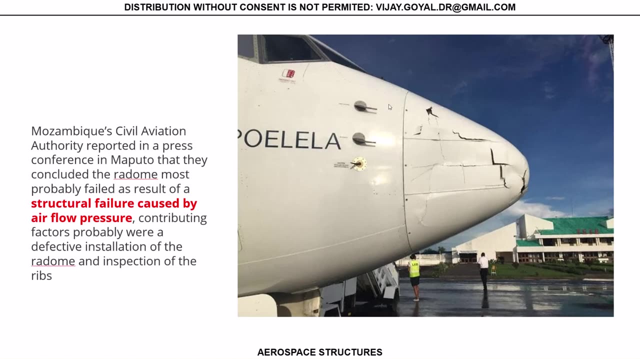 you can see on this section right here. let me change the color. um, do you see wrinkles? there are lots of wrinkles there. that's, uh, that's what we call the skin buckle in that section. um, this is another example in which you may see an airplane like this and you might get freaked out like what happened: got burst. 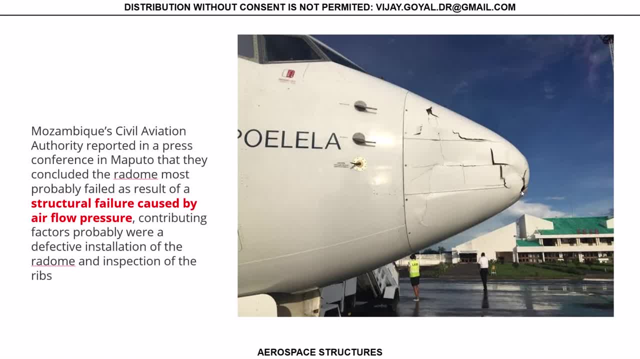 strikes. actually it was not board strike. you're a structural failure because the ribs on the inside, the hold or everything in place that collapsed, so the pressure was higher and actually made it fail. so when your airplane lands and they look at stuff like this, first of all you should be thankful that. 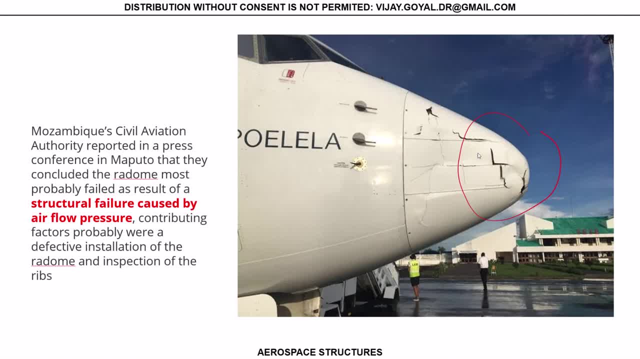 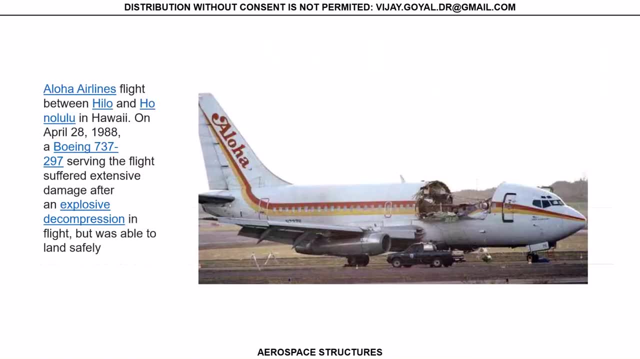 nothing happened to the plane. secondly, you have to ground the plane and repair it. um, we cannot get around that. that is very important. a very typical case. uh, a couple people died in this accident. it was 1988 Aloha Airlines and what really happened was: um, along the rivets. the rivets start peeling. 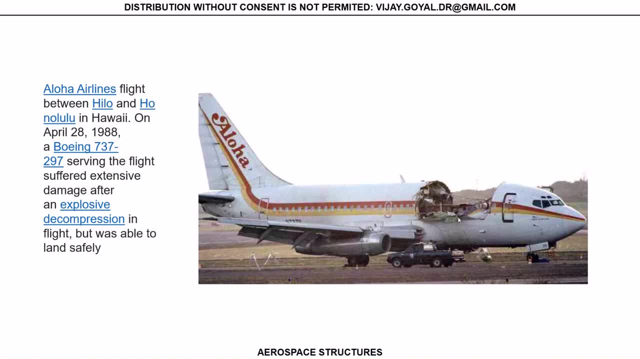 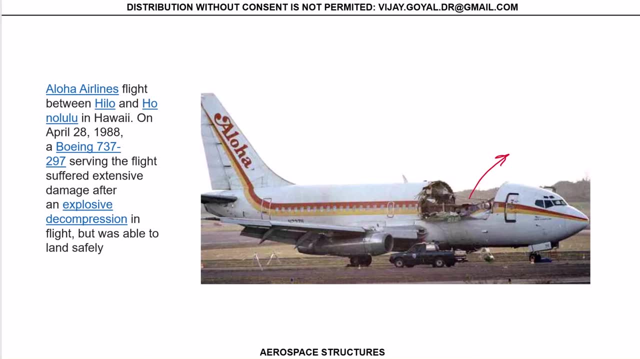 off. so one peeled off, the other peeled off and eventually the whole thing peeled off and the whole upper section just flipped apart, right. and so these are important considerations that we take in the designing planes we want. we definitely don't want that to happen, and history teaches us many of 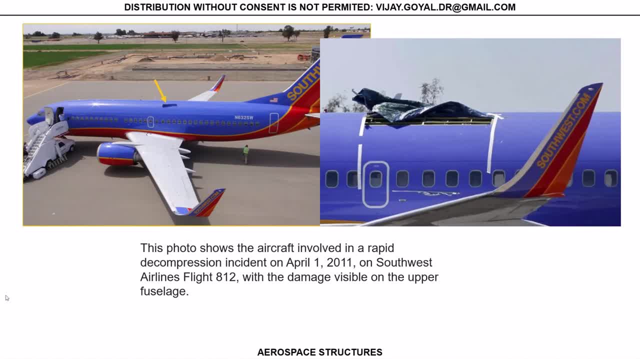 these lessons? uh. this is a more recent um recent uh failure that we saw. this is in uh 2011.. um, this is Southwest Airlines. it's a Boeing, uh a plane, and you can see that during the real flight time, this part really ripped apart and there are some other minor damages. 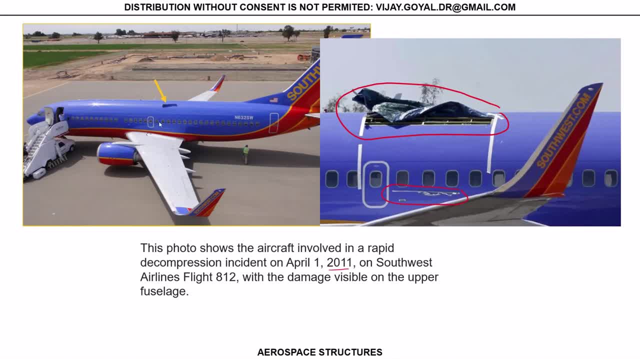 that actually occurred in the plane itself. um, you cannot. yeah, you can probably observe, you can see them here and this is the same. you know, this is a zoomed out view of what this really looks like and you don't want this in a plane, a real flight. you don't, definitely don't want it. but if it does, 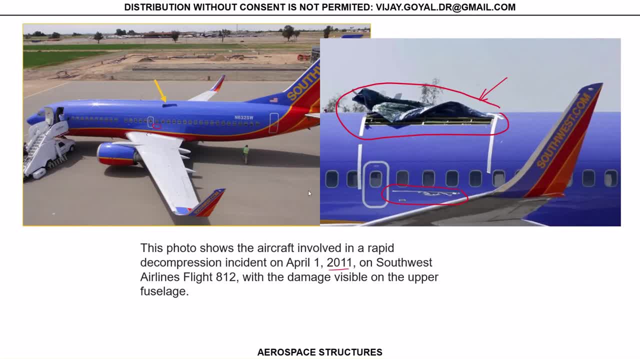 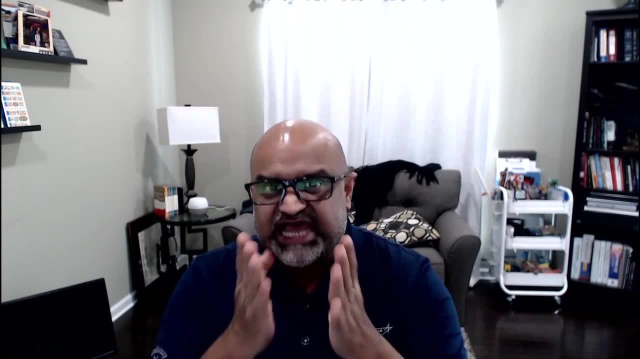 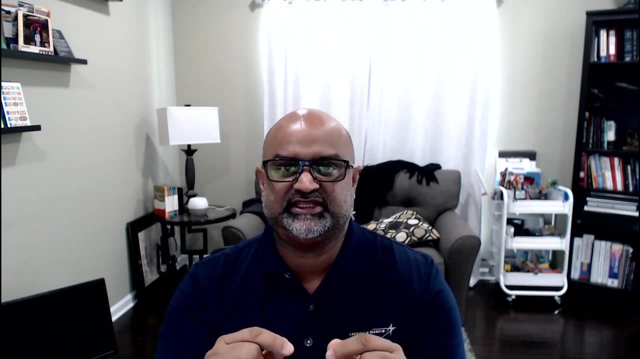 happen. we have to design it so such that, um, we design a plane. so this is very different from every other uh structure that you design. here. we design a plane and we say, if it's going to fail, this is how it's going to fail. I want to make sure they fail such that it fails safe. I want. 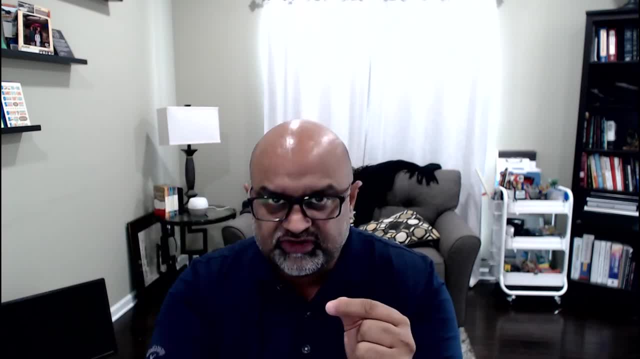 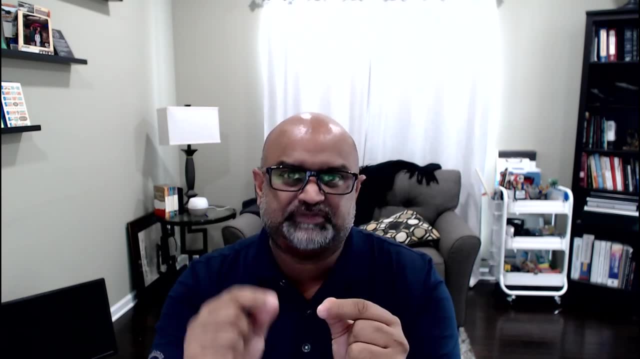 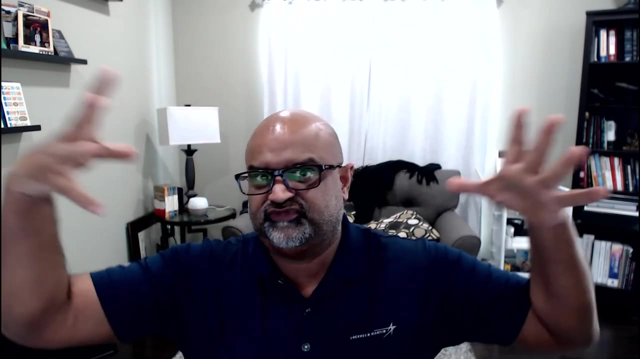 people to be able to be safe. I care for the security of the people, safety of the people, um. so we have to intentionally design what your primary structure is, your secondary load path is, and say, if there's a failure, I want it to fail here, I don't want it to fail the whole thing. 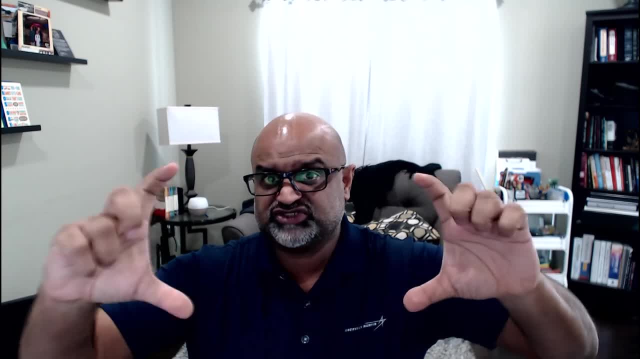 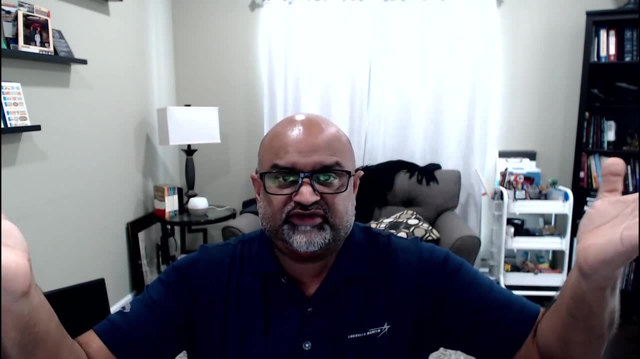 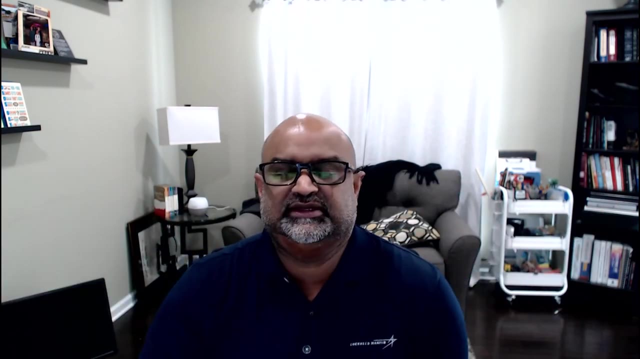 right. so if you got the whole wing box and the wing box fails in the main spar, rear or leading spar, and you have those spars that fail, you lost your aircraft. but if it fails in your mid spar, then okay, I can still drive and maneuver to land my plane. so 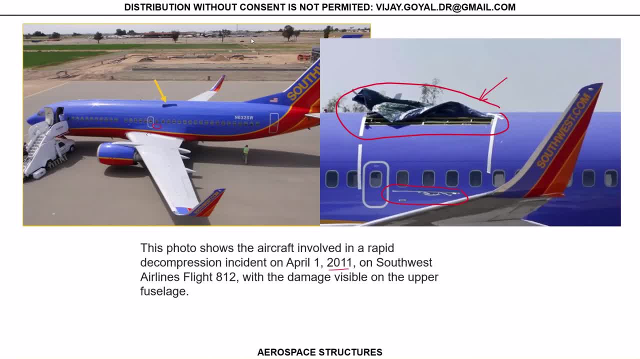 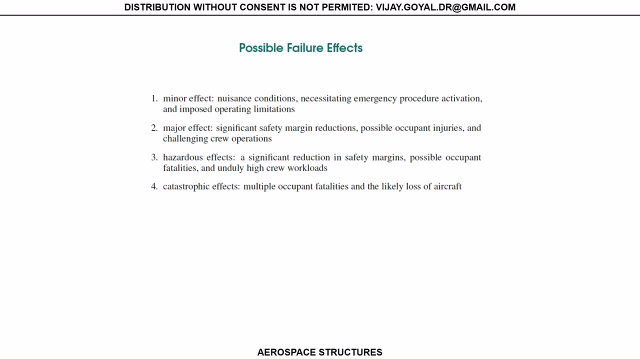 we have lots of inspections that go on between flights, um- or at least they should- and a typical airplane does have a couple cracks, and those cracks are measured to make sure they're below some critical uh, critical, uh- a fracture length. and later on in this class we will teach you how to do that. 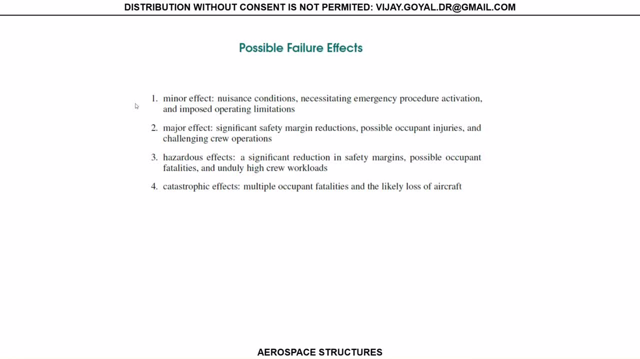 um, basically, a possible case is a failure. these are when the minor effects, the major effects, um, is what we really? you know, we get freaked out any of this- uh, the hazardous effects, um, and then you get catastrophic effects, right, these are when you lost your aircraft and their 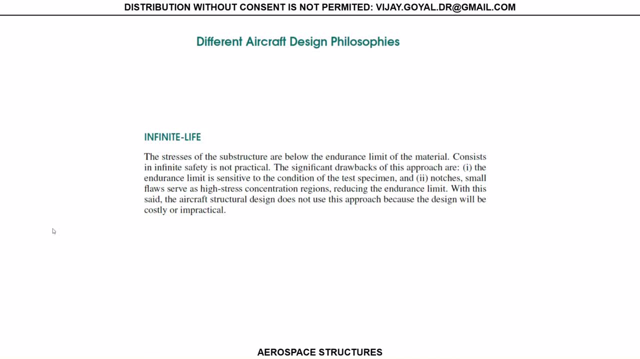 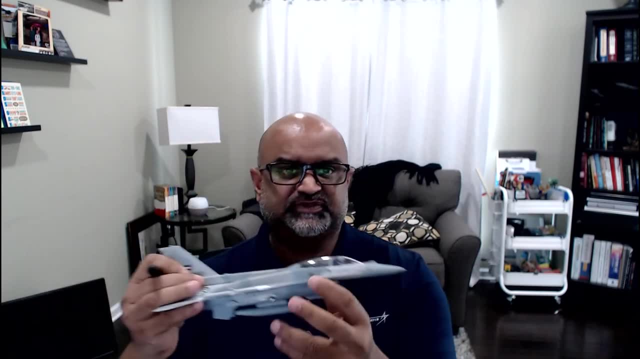 casualty. um, take a couple designs. the first of design is infinite life. will you design a structure? as you can imagine, I will design a plane and it will say: this plane is going to last me forever. uh, you don't want that at all. you don't want to plane. 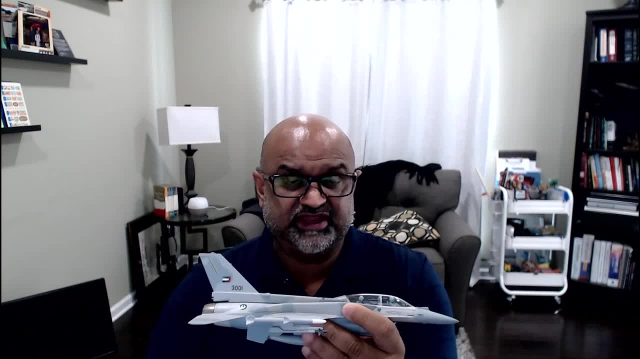 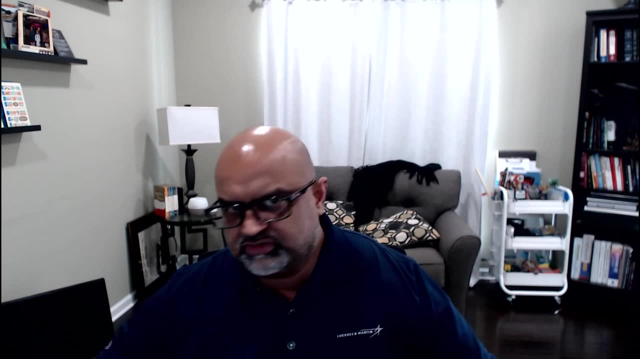 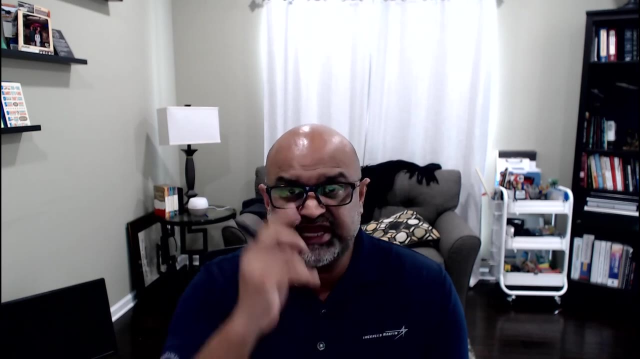 to last you forever. why? because it's going to be costly, heavy the materials you're going to use. so you design a plane. that's one way to design it and some few applications. maybe there's a case where you want to design an Infinite plane, but you Infinite Life plane, but you don't. you design a. 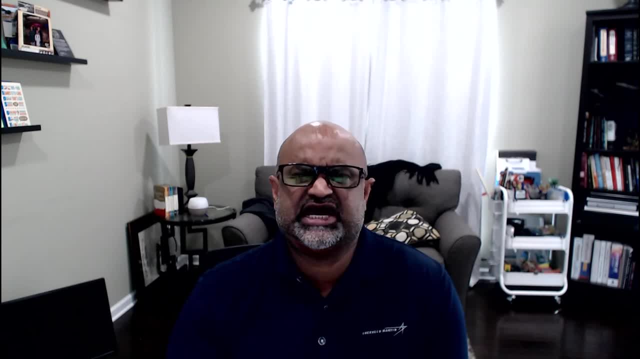 mainly for certain service criteria. it may be designed for 20 years of life and we are done with the plane. 30 years of life and we are done with the plane. now there's a different philosophy, or depending on who is buying the plane, like, for instance, commercial aircraft, they will buy a plane that typically has a lifespan of 25, 20, 25 years, but they will keep on doing repairs and those repairs that can take the plane up to 30, 35 maybe, maybe years and they have and but the repairs are not cheap. they're very expensive as well. so it's a trade-off in terms of when you stop. when you stop repairing and say it's time to replace the fleet, okay, in the Navy, we care. Navy cares for designing me a plane for 20 years. after that dump it, I don't care for it. Air Force, on the other hand, 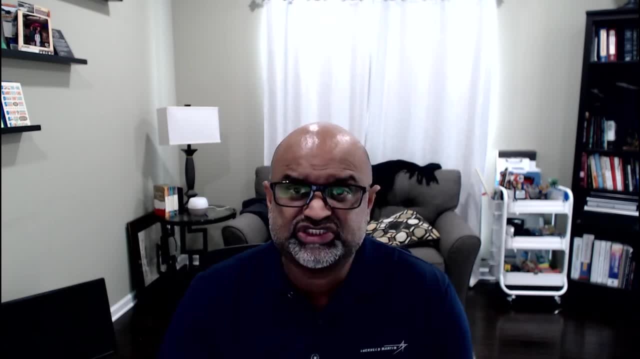 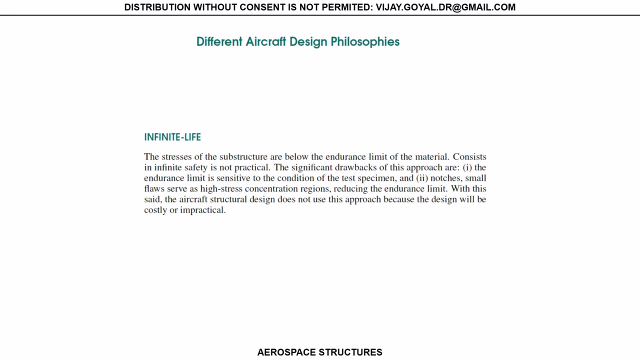 they care for damage. that damage tolerance, in which they care for. if I can get five more years from the plane, two more years I will. so the philosophy is different for both of them. then you design a plane for their gear, towards their needs, okay. so, with that said, the 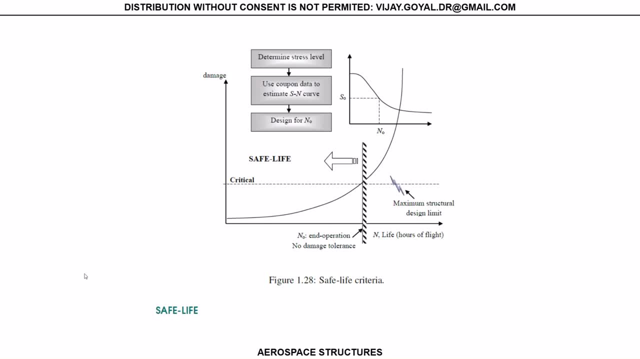 second criteria is the safe life criteria. we are basically saying that, well, there is a damage in your problem in your aircraft and that damage is going to be given. that damage is located right anytime over here. so if I have a damage, it doesn't reach my critical damage criteria, so I can still fly my aircraft. 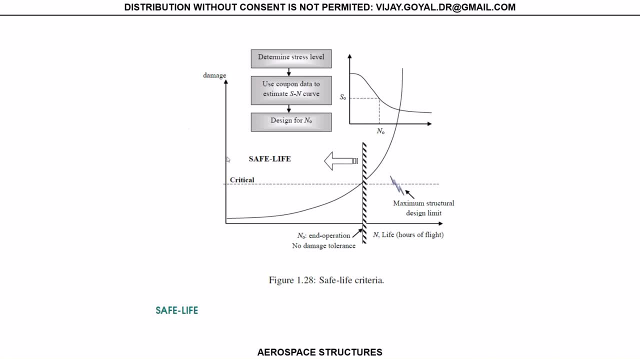 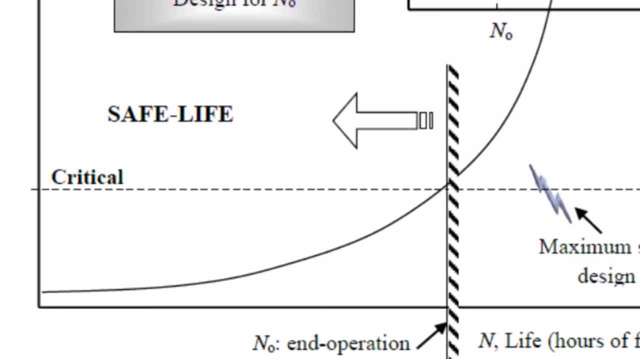 and I want to make sure as to- I'm not sure if you can appreciate this, but let me see if I can zoom this so you can really appreciate this. so when it hits this, this mark right here is still: it's not failed. he has not failed at all. okay. 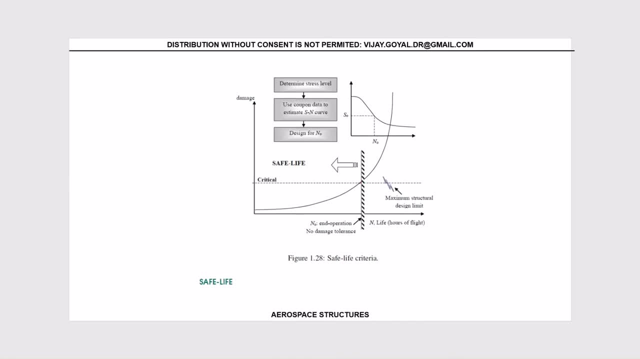 um, so that's what we want to do. it we want to make sure that if there's a end, there's a cut off, that you want to take technical situation and you want to stay below the critical and after that you just dump the airplane. you don't need. 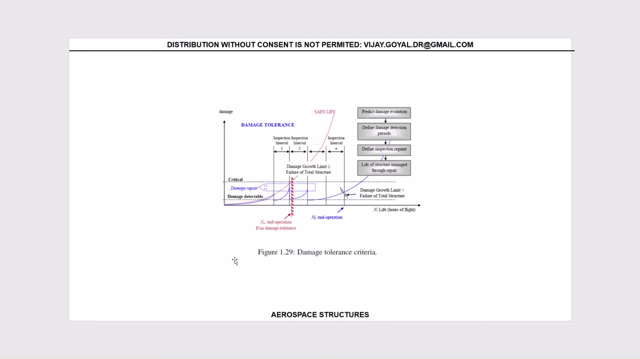 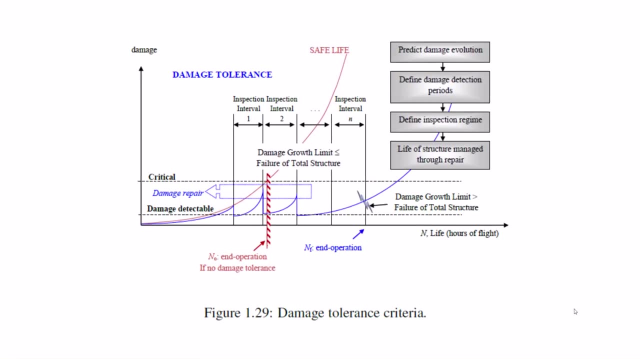 the airplane anymore. damage tolerance, on the other hand, is very different, because damage tolerance is based on constant, a constant inspection, and if there's a damage and we can repair that damage, we try to repair it and bring it down to a here, and then we constantly are repairing and repairing and repairing, and this will be the. 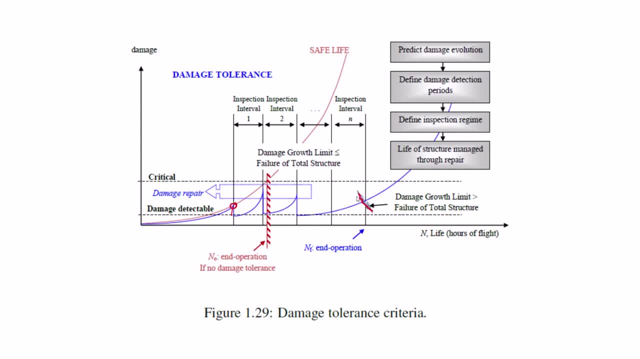 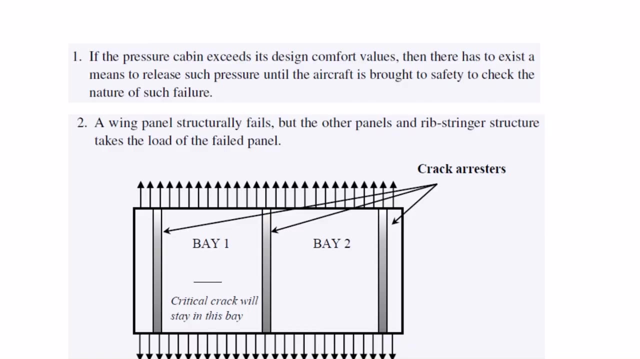 location in which i i can no longer repair my airplane, um, but i will stop. have a cutoff somewhere over here after many, many, many different damage, uh, damage criterias, um, but the trade-off with this cry with damage tolerance now, is you need to create a secondary load path. as for an 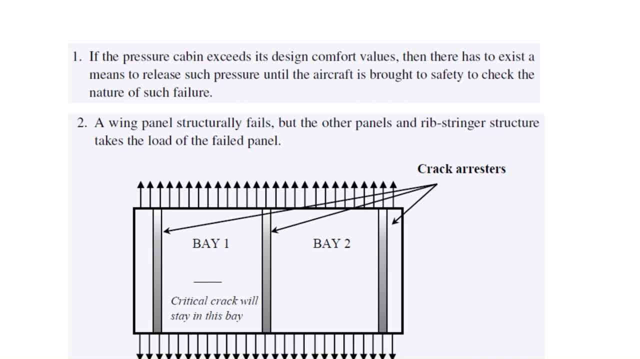 example, i wanted to consider the uh pressure cabin of an airplane. uh, it's comfort, it's comfortable. but what happens if the airplane actually- uh, there's a pressure problem? well then, there is a pressurized uh. there is a mechanism to actually address that issue within the plane. let's suppose 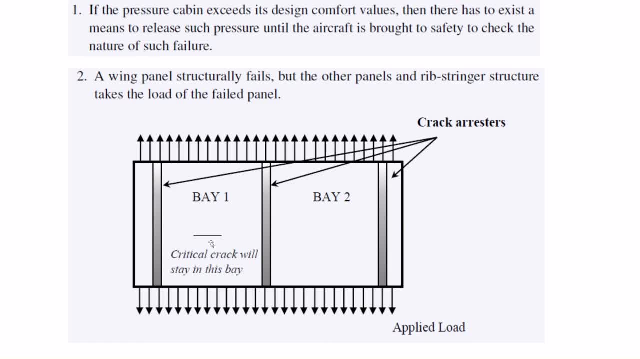 they got two bays. this pay that has a crack in it. well, if this does have a crack, i want to create this load pass i so if you would. i lost this plane. i lost this panel because of of this crack, so this can no longer hold the load. 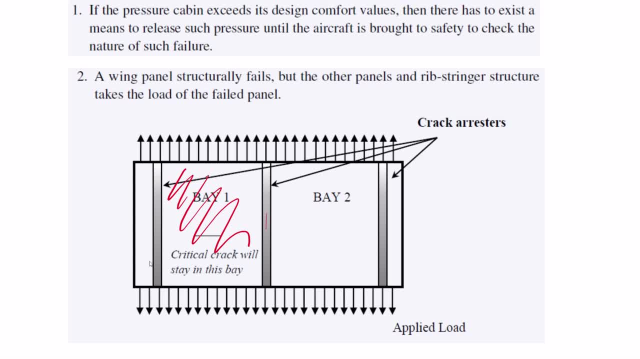 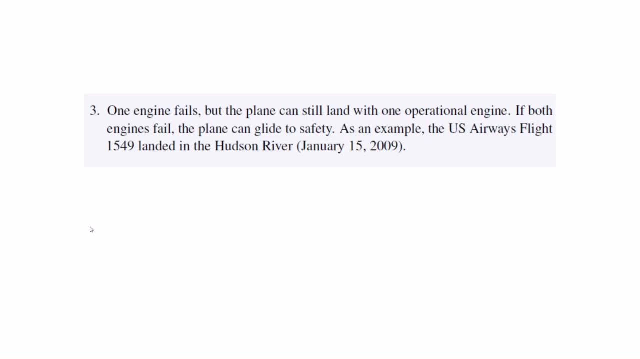 but can these two crack arresters hold enough load to make my plane land, and so i can repair this later. so these are the different things that you have to keep in mind when we're designing planes. another very interesting case is what happens when we have two engines. typically, a typical airplane has two engines, and the reason behind it has. 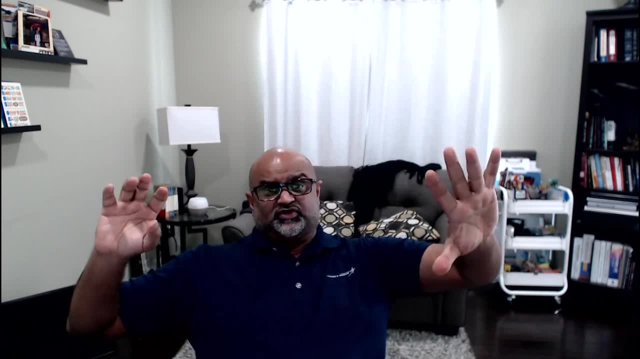 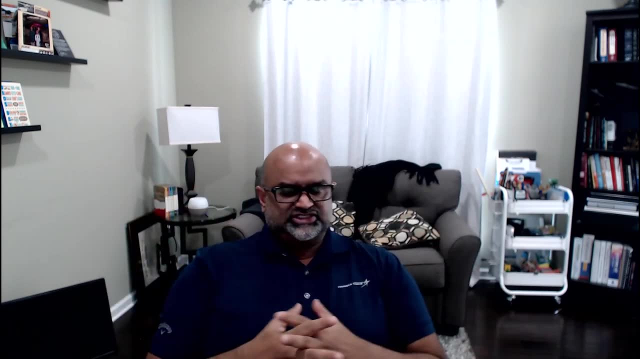 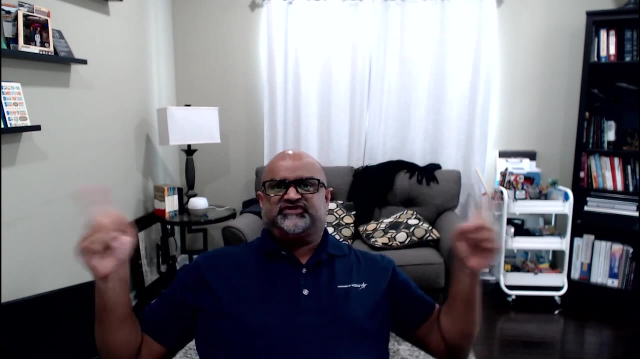 two engines says if one engine fails you can fly with the second one. the extreme case is the case of the hudson river. not sure if you read it or you heard about that in the history books, um, but that plane was very phenomenal because, uh you, both engines failed. 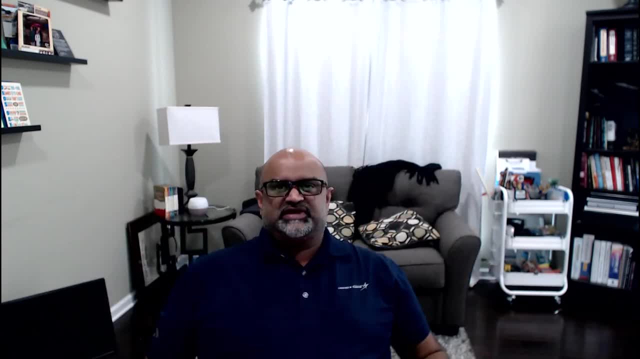 and the pilot has a matter of seconds to make a decision. do i try to turn and land the landing water? what do i do? he sees the hudson river and then he says i'm going to land in the, just wait for me there, and he makes a very awesome landing. that's actually everything goes. 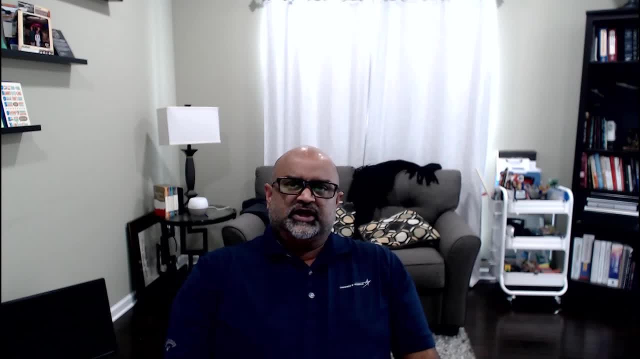 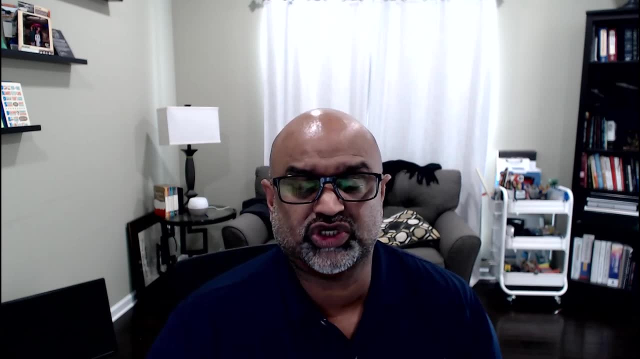 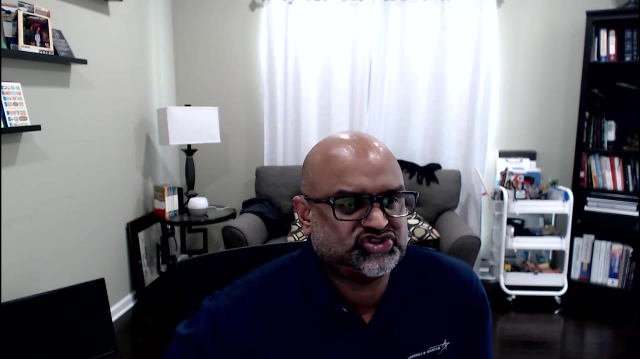 in such a case you have to give credit to um, to the pilot, uh and and, and. thank god, thank god that you didn't have any other further structural failure in which your plane was actually able to land. so we aerospace engineers- uh, airspace structural engineers- are responsible to design. 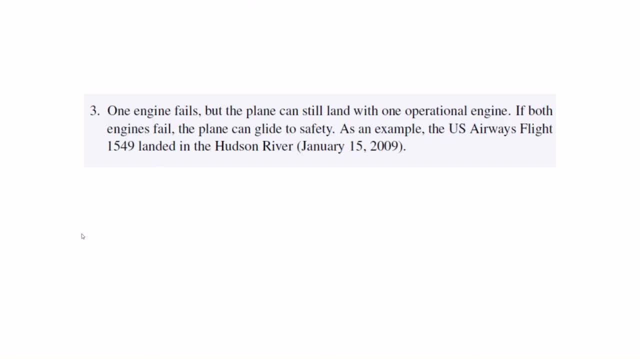 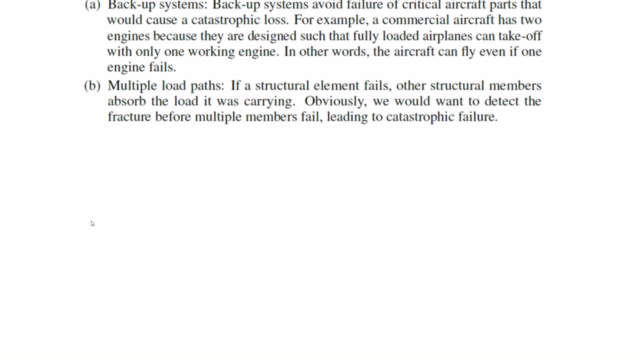 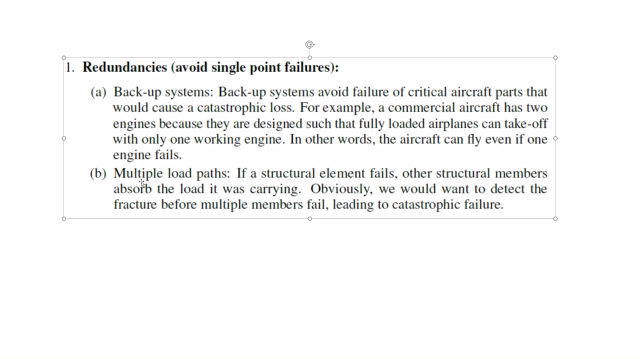 planes, uh, such that they will be safe in every possible circumstance. okay, so, um so, we have what we call multiple, we got the backup systems and we have multiple load paths. we don't want to rely only on one load path. that's why we have more than one spar, more than one rib if one fails my 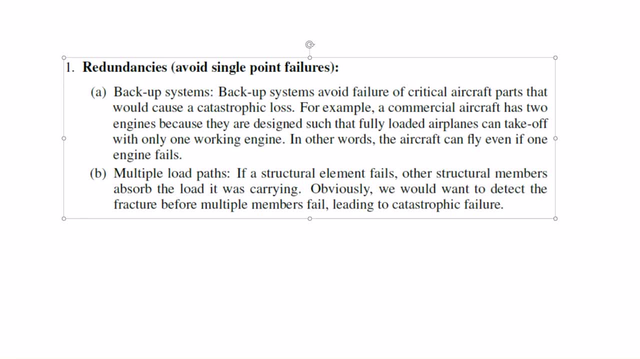 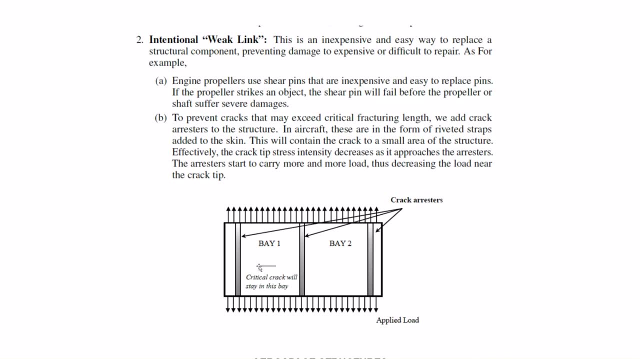 plane, the whole plane can still fly. um, and then, as well, we have crack arresters right, because we want to make sure the weakest link will be the bay and i will let it fail. so if it's going to fail, i make the path and i design this so you fail. 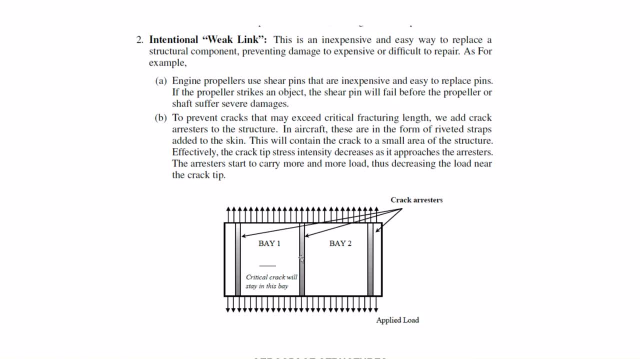 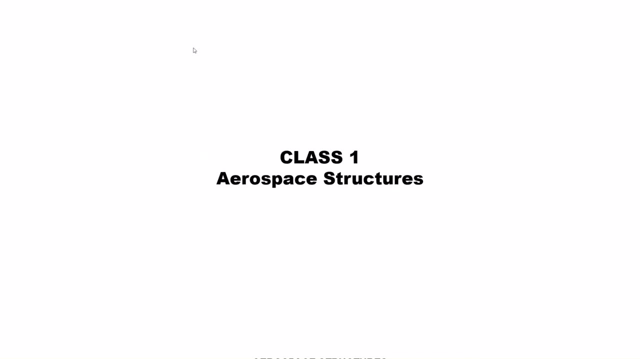 here and not fail over here. okay, so these are some criterias that we keep in mind when we are designing airspace structures and throughout the course, that's what we will try to um uh, how do we design strong while keeping light airspace uh structures, uh to make uh robust airplanes? that's going to be the focus of this course.